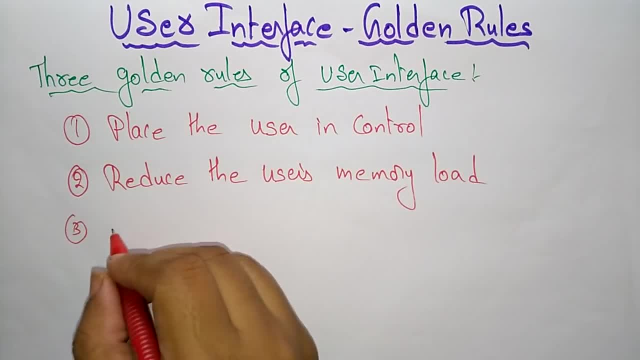 And the third one is: make the interface consistent. Make the interface consistent. So these are the three main golden rules that we have to follow in the case of user interface. So the user interface has to place the user in control First. they have to place whatever the user that we are going to be used, that user has to be in control. 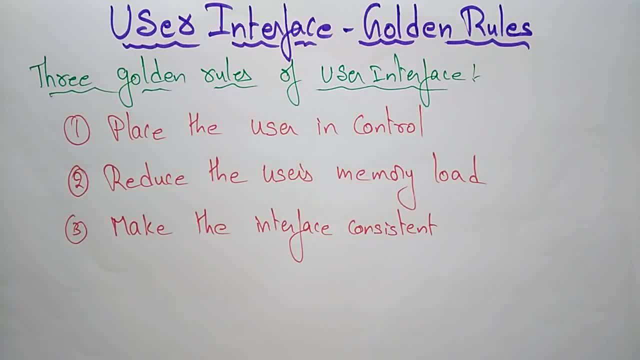 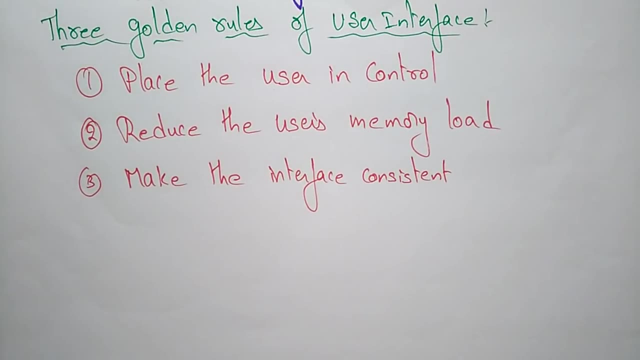 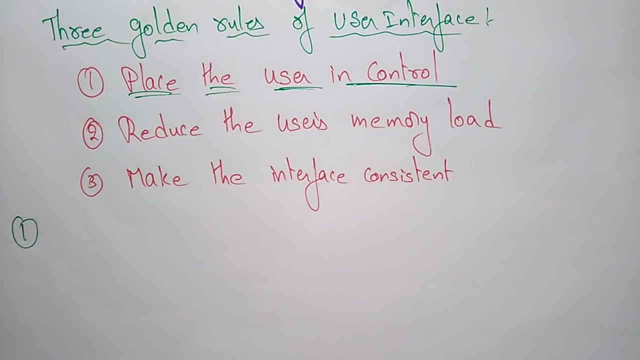 And the third one is: reduce the user's memory load. So, whatever the app we are designing and whatever the product that we are designing, So the main thing is we have to reduce the memory load on users and make the interface consistent. Okay, now let us see in detail what is the first golden rule, that is, a place the user in control. So what this? how we can place the user in control? What are the techniques we have to follow to place the user in control? 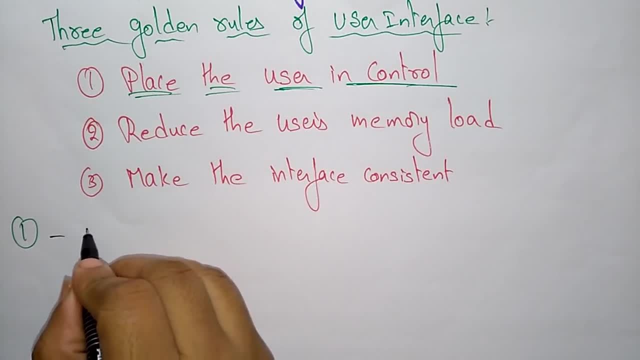 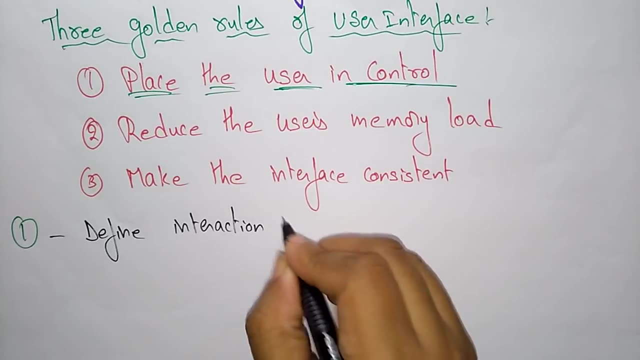 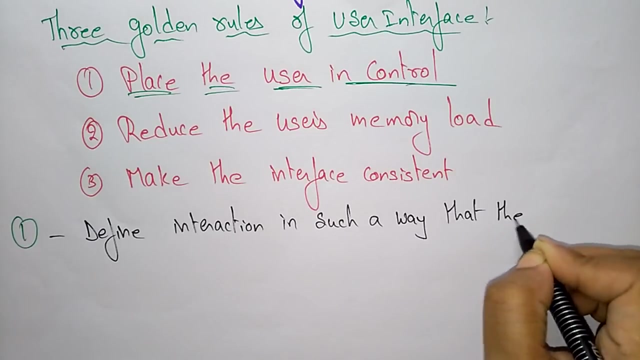 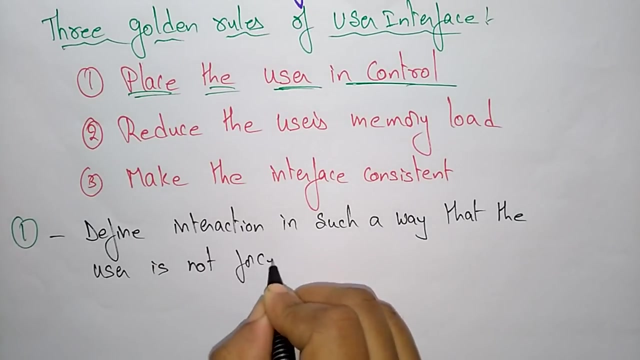 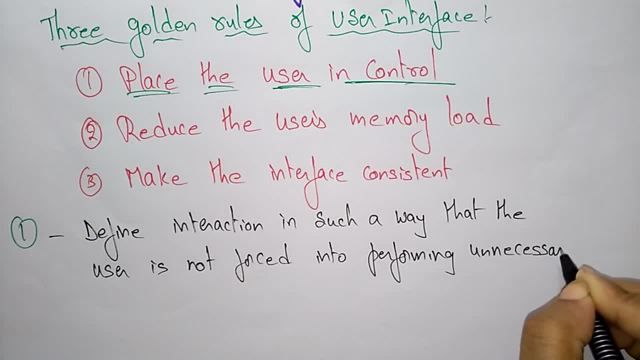 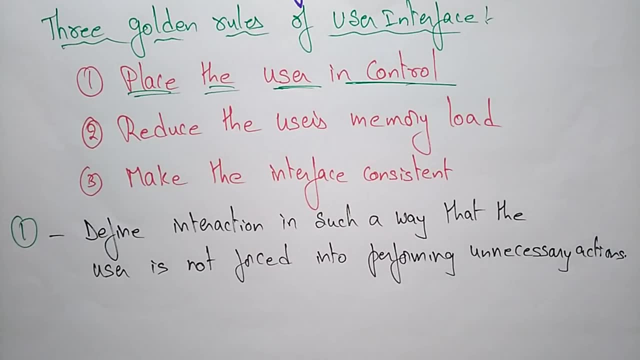 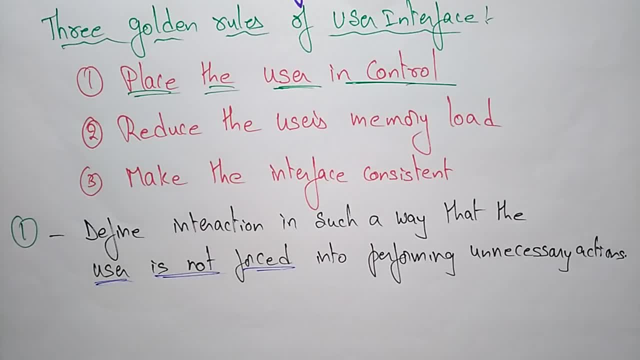 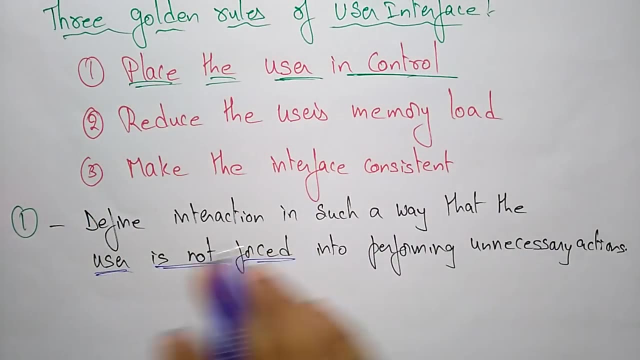 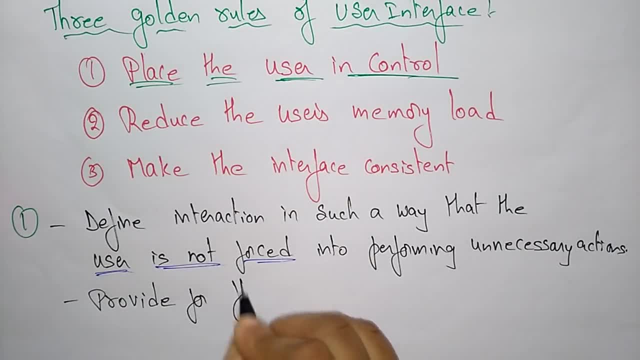 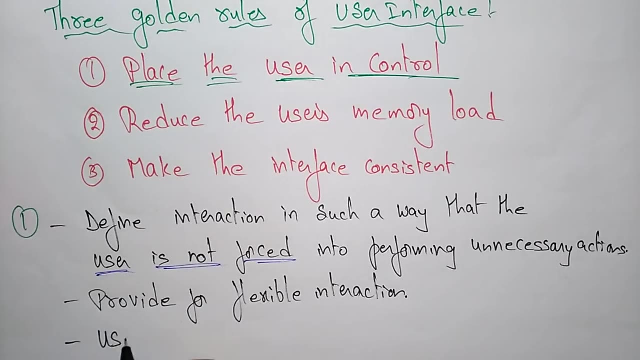 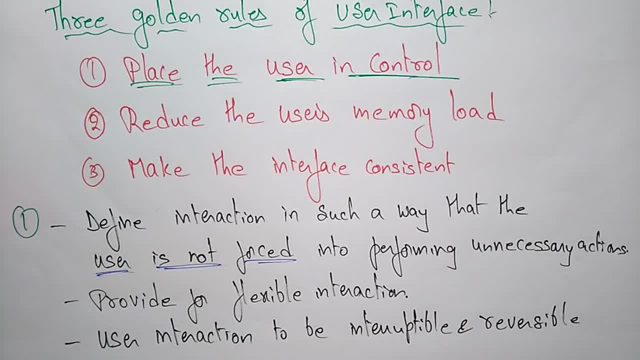 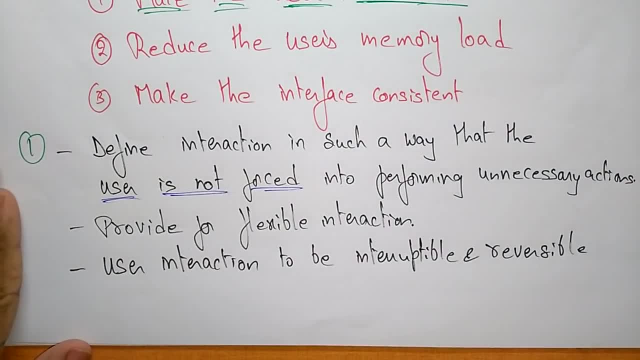 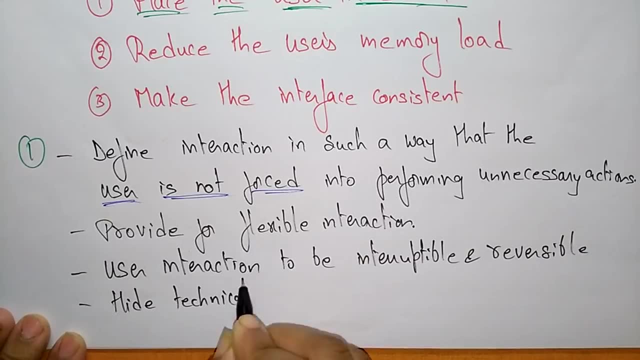 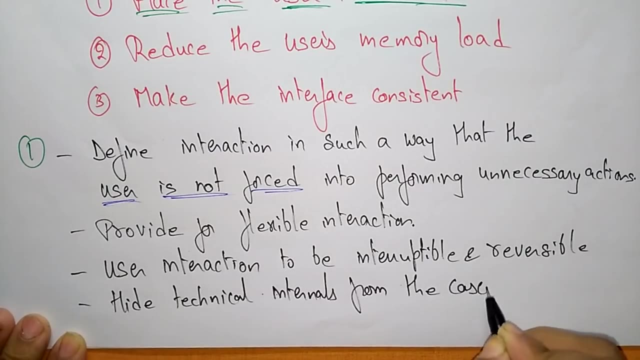 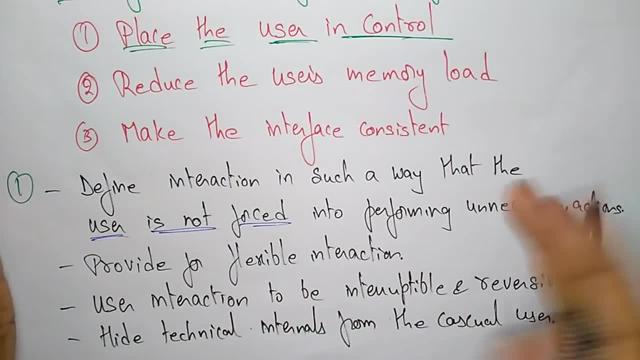 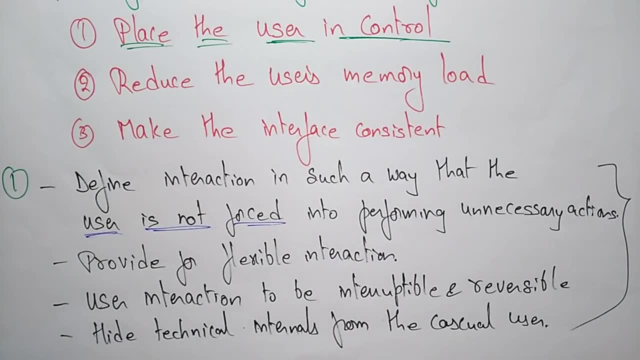 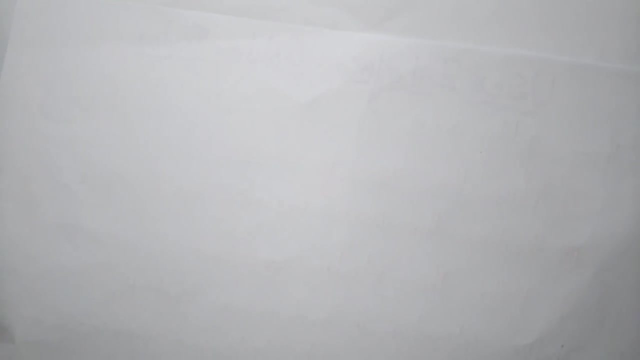 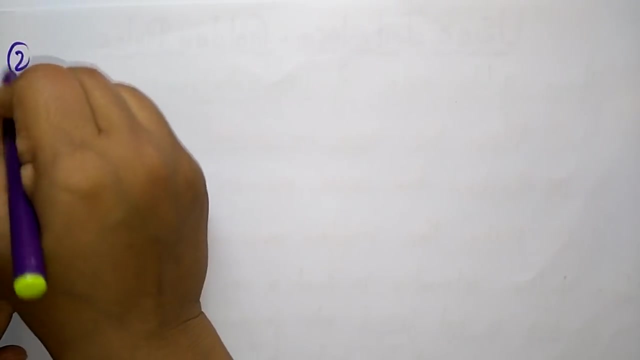 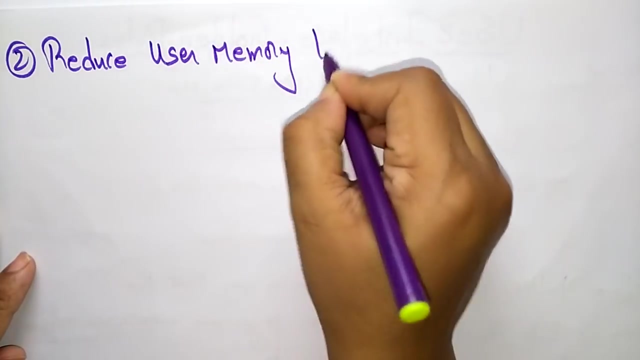 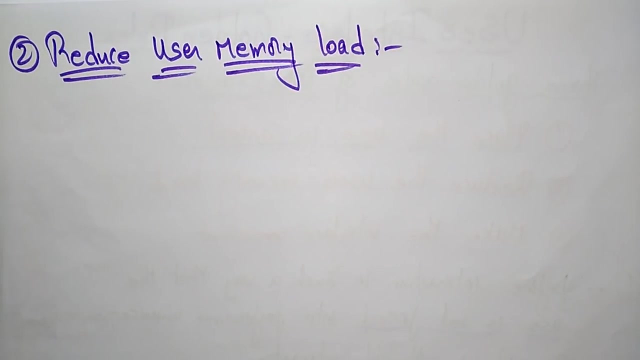 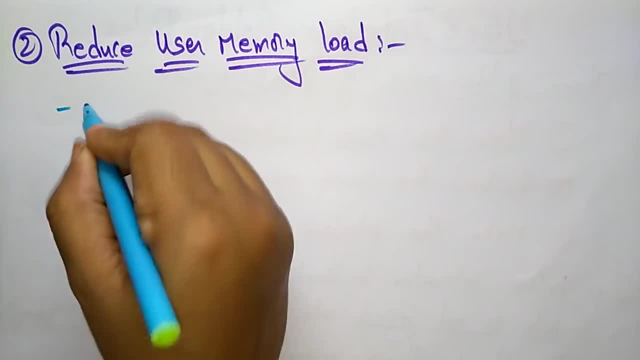 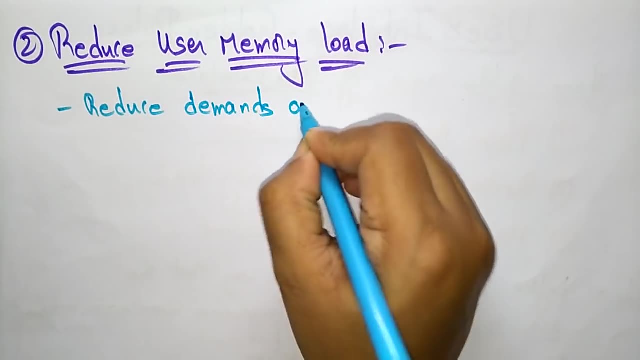 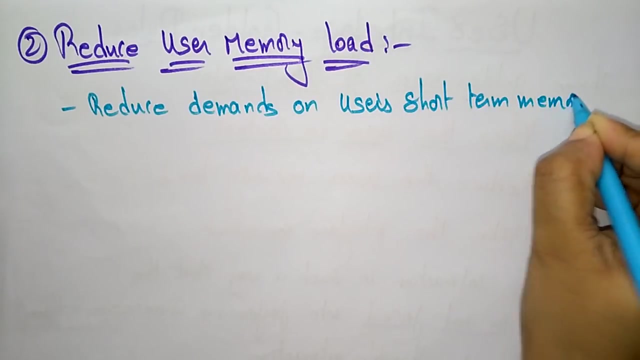 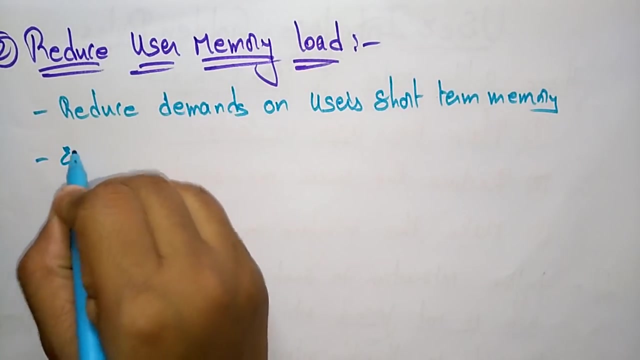 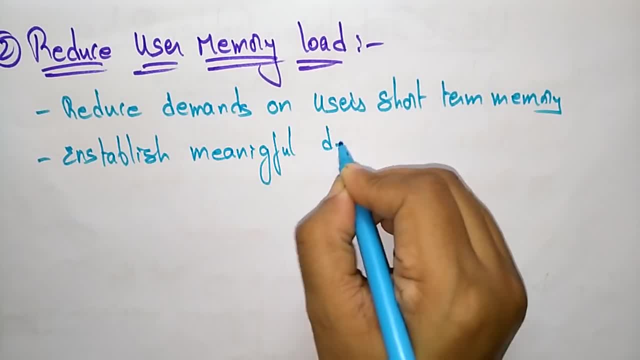 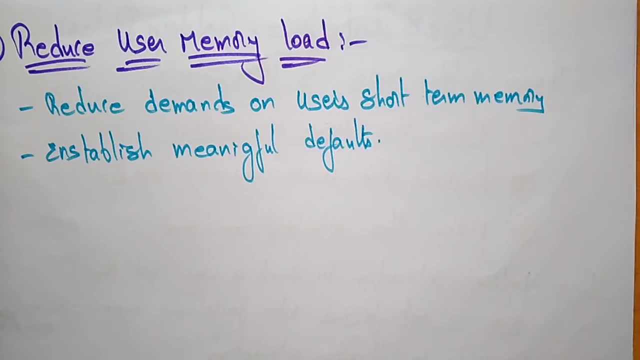 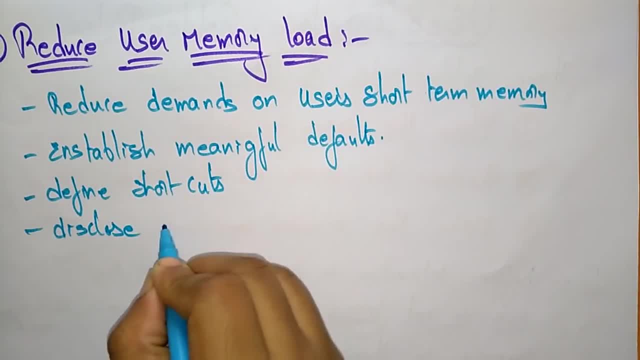 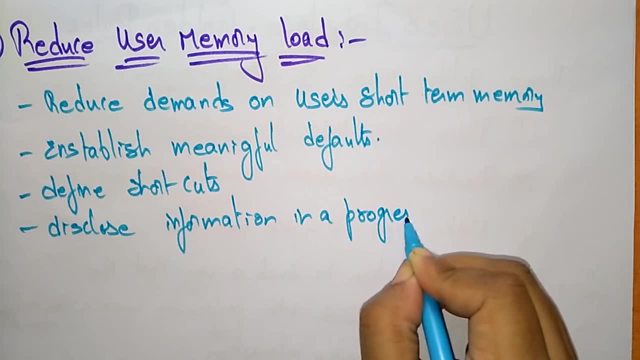 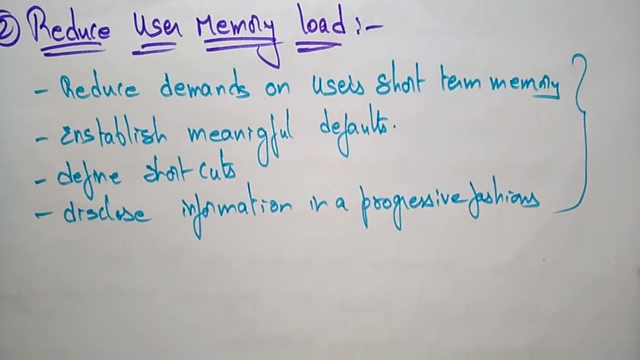 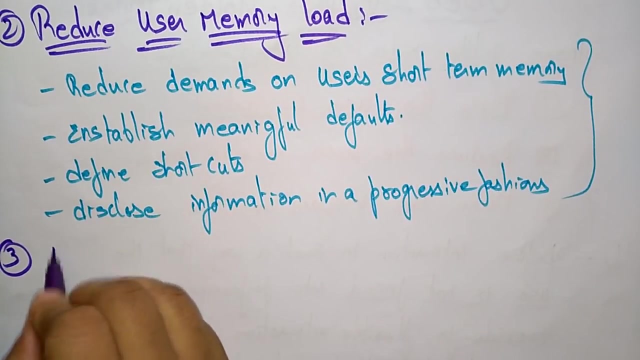 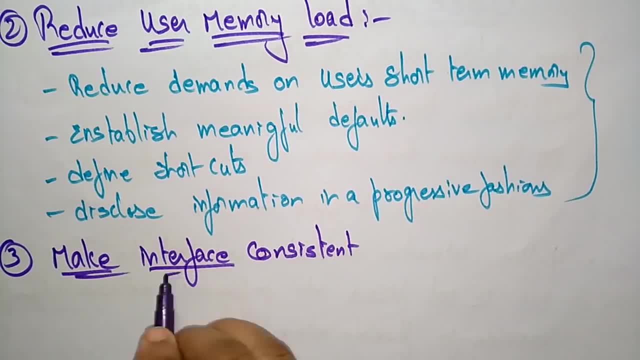 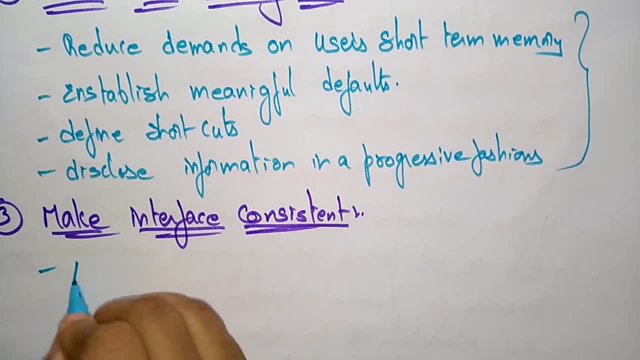 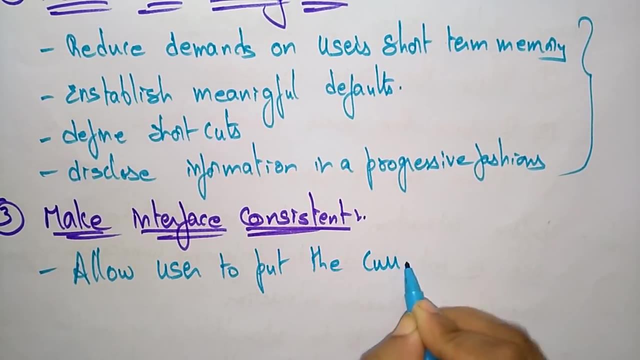 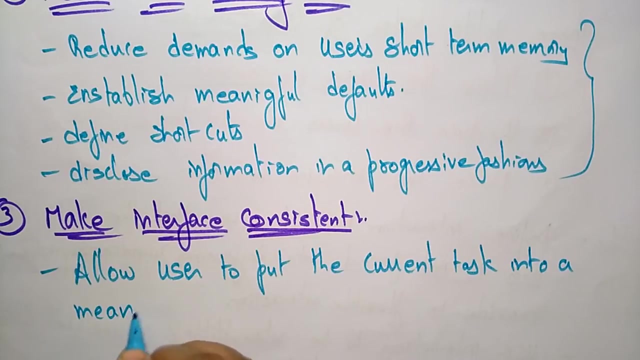 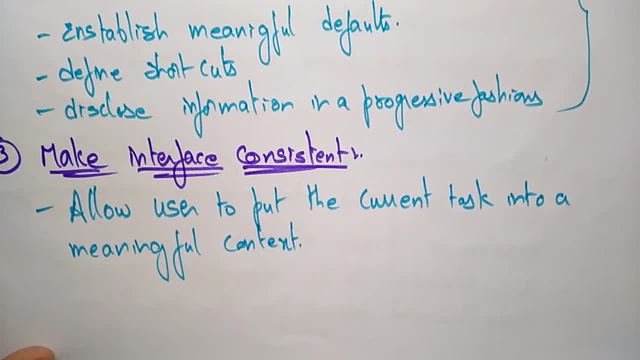 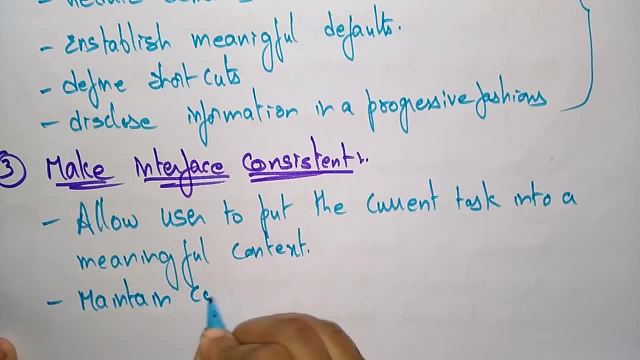 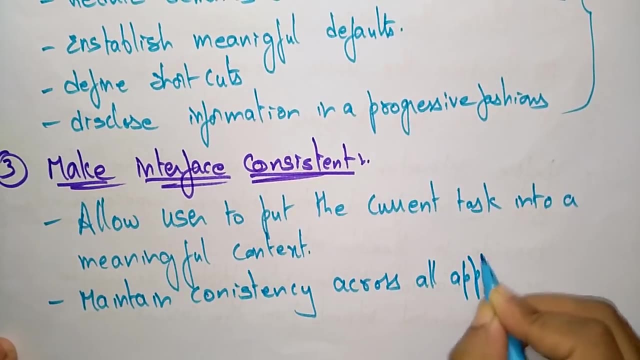 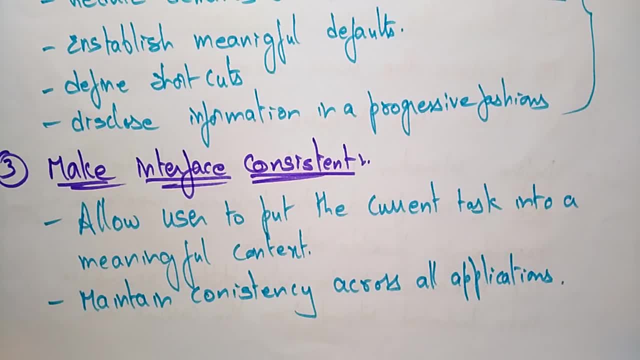 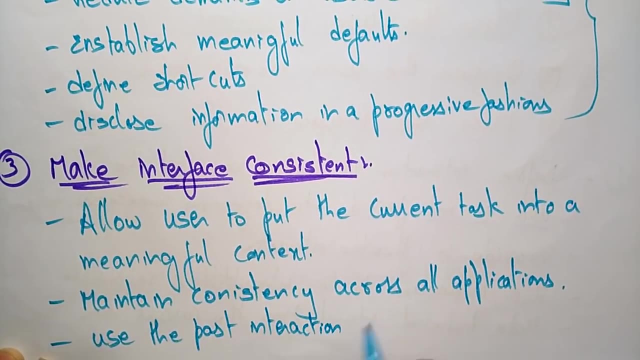 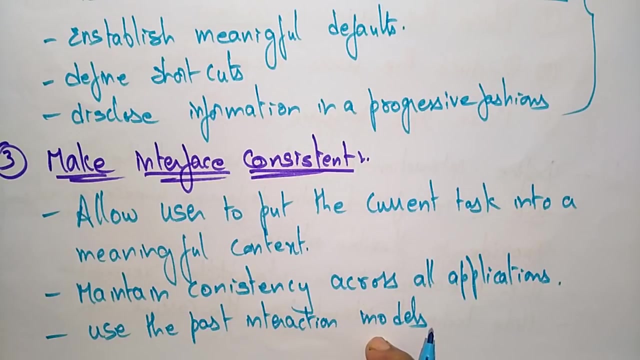 fist define interaction in such a way that the user is not forced into performing the actions. So, because they are already proven, that models are already proven- uh, the consistent state, so try to use that. so, suppose, if you want to make any changes to that already created past? 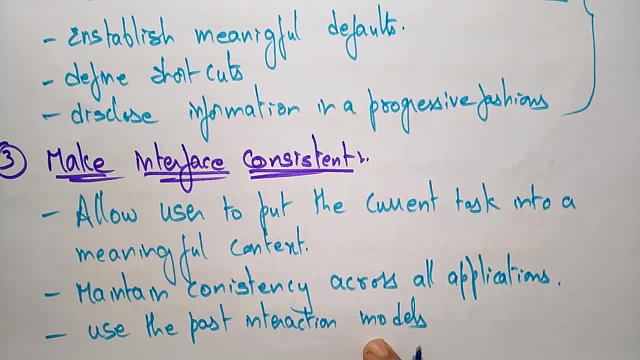 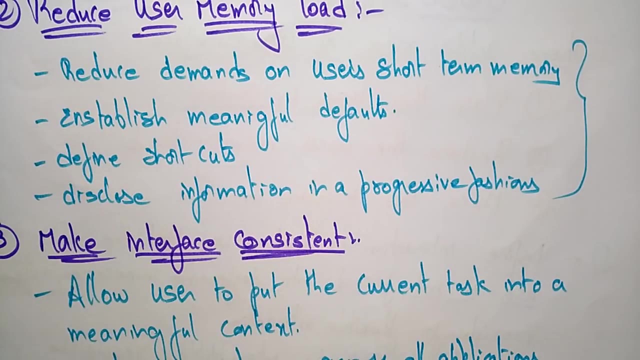 interaction models. until there is no good reason you can't, you don't change. okay, do not make changes unless there is good reason to do so. so these are the three main golden rules of user interface. first, place the user in control. second, reduce the user memory load. 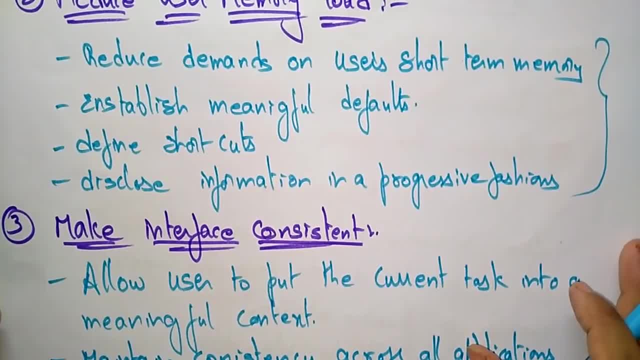 and third one is make interface consistency. thank you.